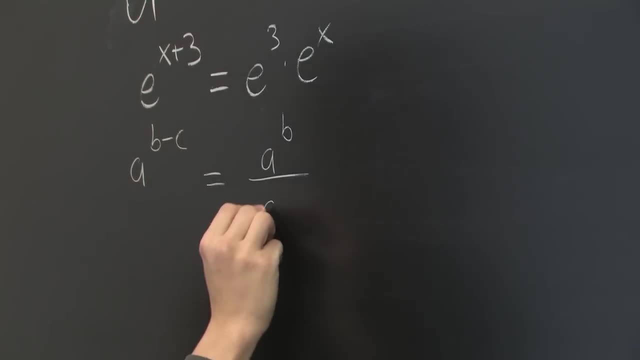 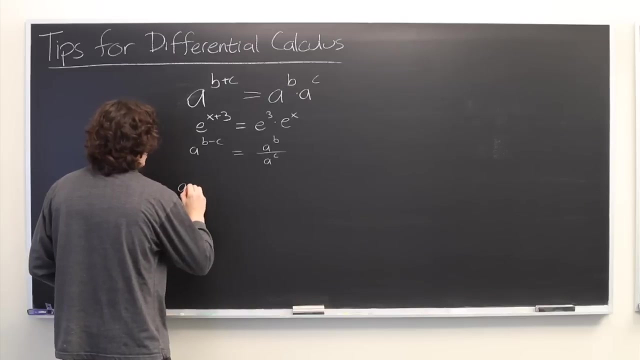 better minds. you've spent two hours here. This seems like a lot of time. So what we're to the b divided by a to the c. Okay, what about logarithms? Let's say you've got something like a times log of b. Well, if you're multiplying a log by some constant a, you can actually 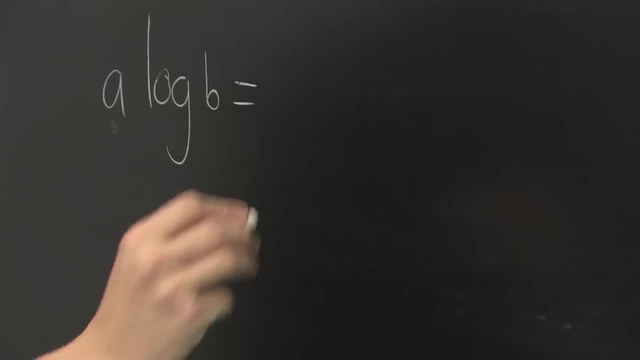 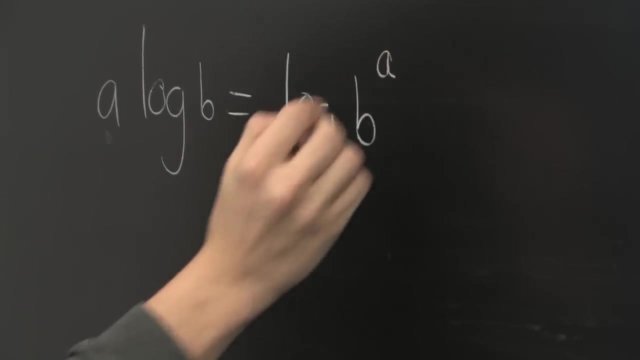 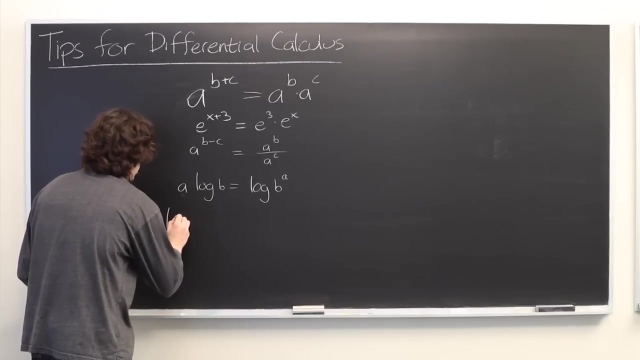 bring that inside and it becomes the exponent of whatever's on the inside. So this becomes log of b to the a-th power. Okay, another useful property of logs, and one that is frequently mis-remembered or simply gotten wrong. Let's say you've got log of a times b. Well, this, 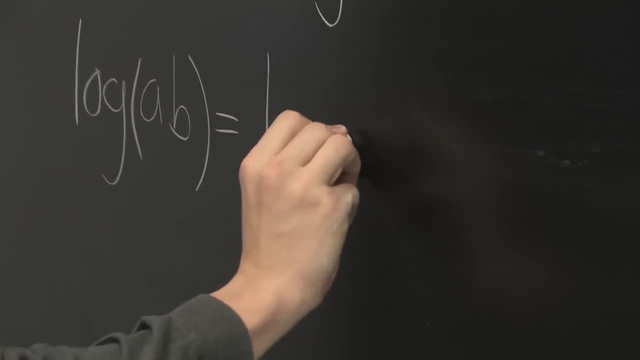 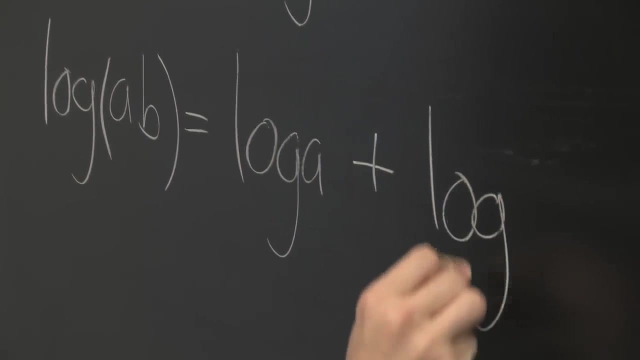 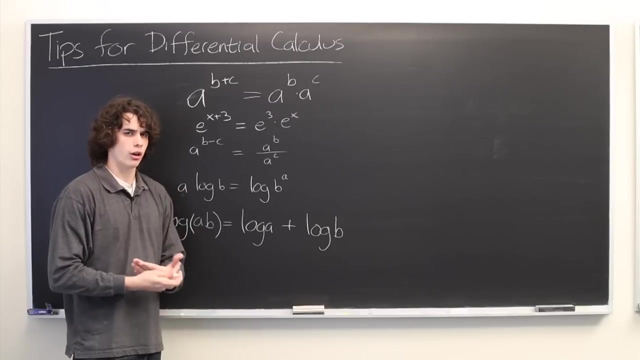 is equivalent to the log of a plus- not times- plus b to the a-th power, The log of b. Okay, so, assuming that you have a strong understanding of the function that you're working with, it's still possible to make a mistake when you're actually applying. 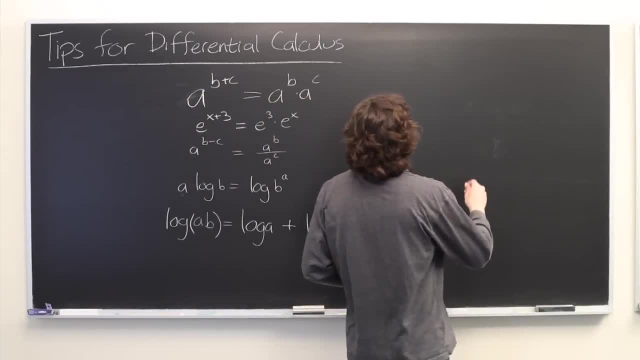 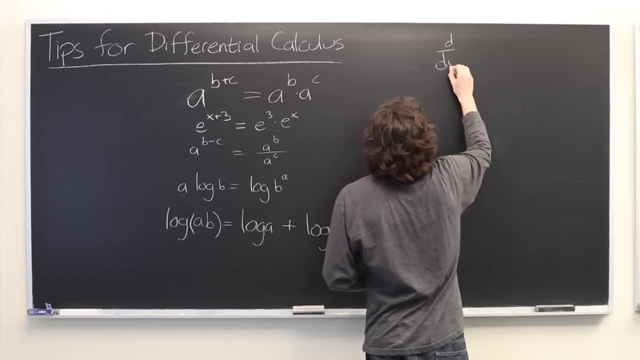 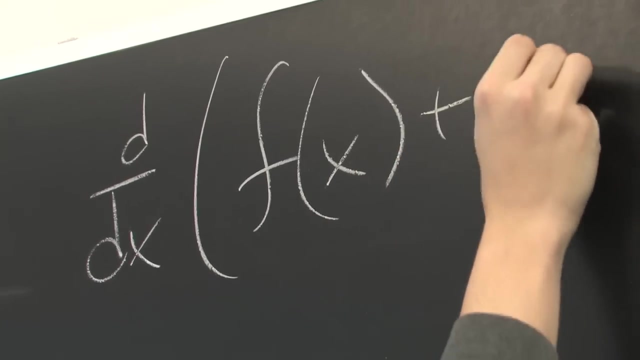 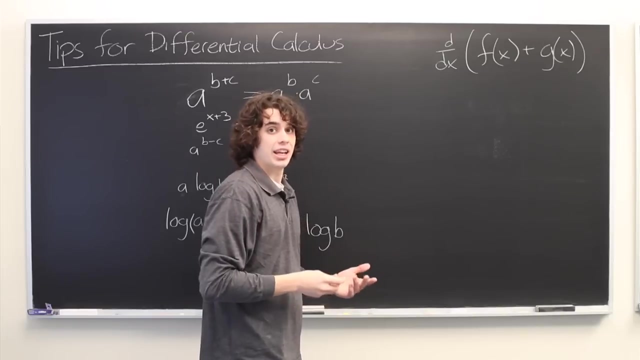 them, For example, when you're taking derivatives. So let's go over some of the helpful properties of derivatives. Let's say taking the derivative with respect to x, of some function of x and plus some other function of x. Well, here we can apply the linearity of the derivative. 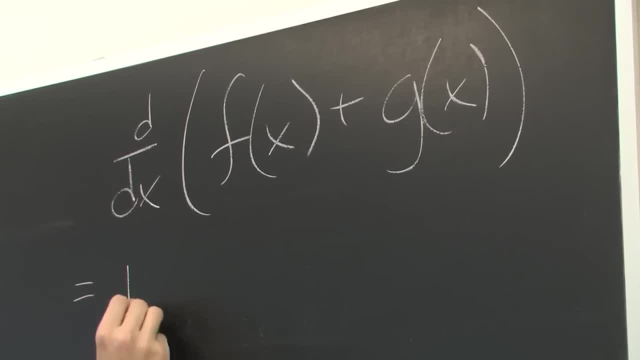 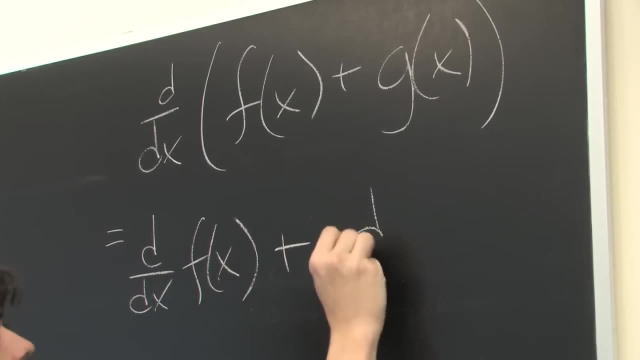 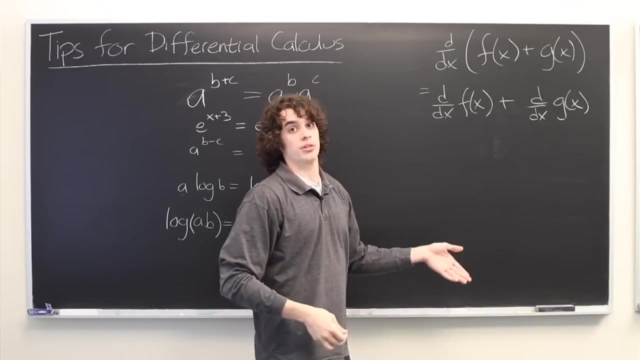 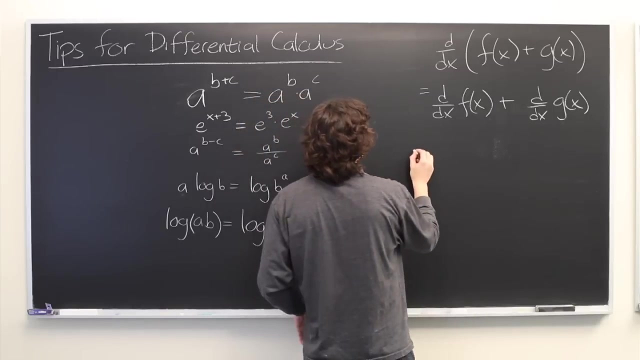 which tells us that this is equivalent to the derivative of f of x plus the derivative of g of x. Or here we might have: f of x equals x squared and g of x equals sine of x. So this works for any functions. But suppose we've got something like this: We have the 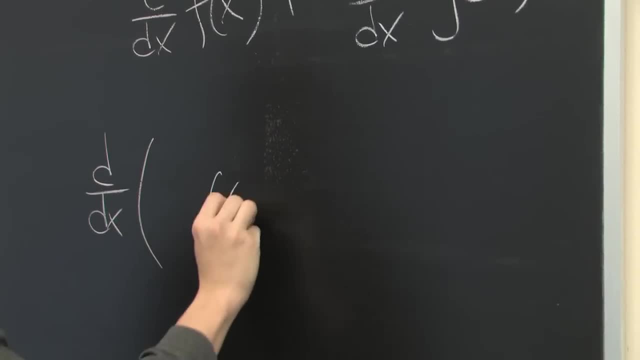 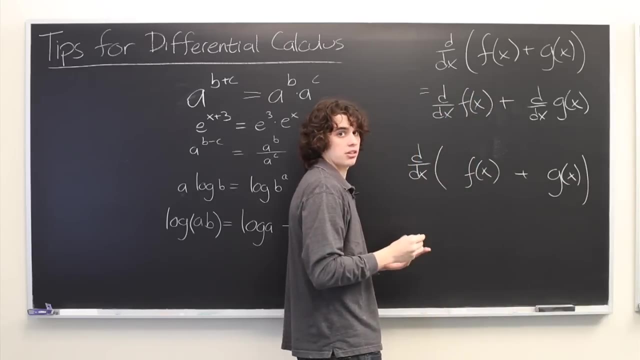 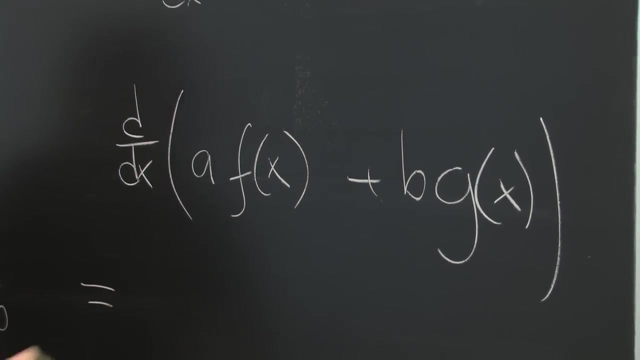 derivative with respect to x. Again, f of x plus g of x. But this time let's say we've got some constants thrown in there. Call them a and b. Again we can apply the linearity of the derivative, which tells us: